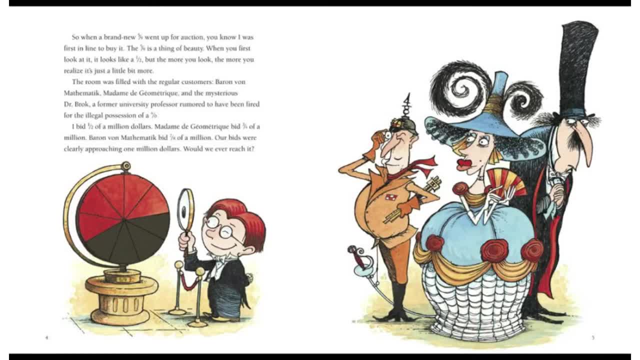 this. The room was filled with the regular customers: Baron von Mathematik, Madame de Geometrique and the mysterious Dr Brock, a former university professor rumored to have been fired for the illegal possession of a four over zero. I bid half a million dollars, Madame de Geometrique. 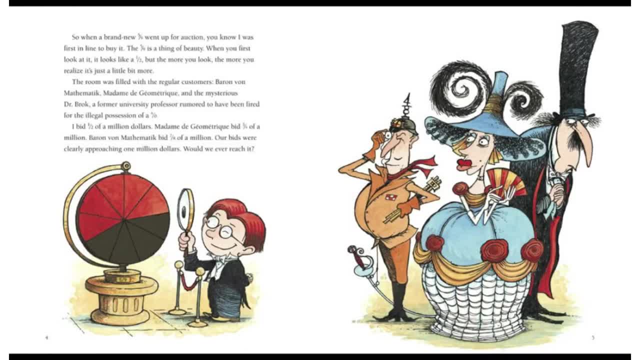 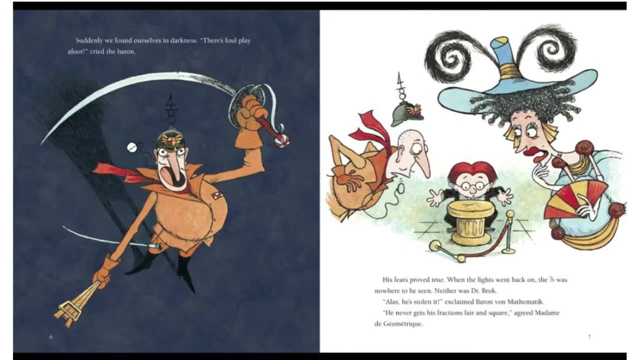 bid three-quarters of a million. Baron von Mathematik bid seven-eighths of a million. Our bids were clearly approaching one million dollars. Would we ever reach it? Suddenly, we found ourselves in darkness. There's foul play afoot, cried the Baron. 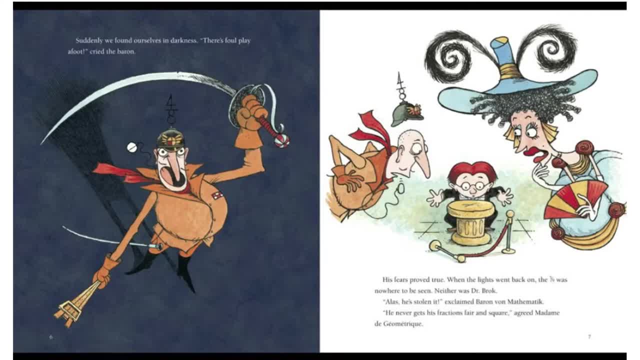 His fears proved true When the lights went back on. the Five Nights was nowhere to be seen. Neither was Dr Brock. Alas, he's stolen it, exclaimed Baron von Mathematik. He never gets his fractions fair and square. agreed, Madame de Geometrique. 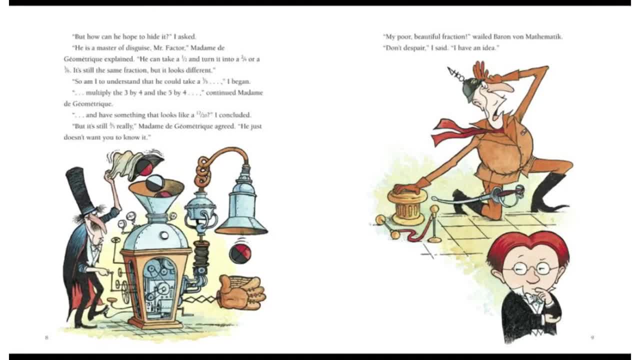 But how can he hope to hide it? I asked. He's a master of disguise, Mr Factor. Madame de Geometrique explained He can take a half and turn it into a two-quarters or a three-sixths, It's still the same fraction. 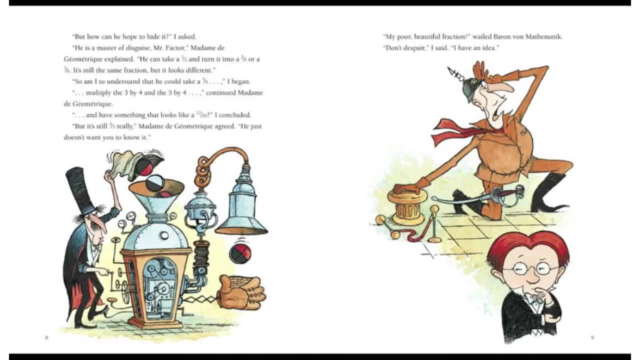 but it looks different. So am I to understand that he could take a three-fifths. I began, multiply the three by four and the five by four, continued, Madame de Geometrique, And have something that looks like a twelve over twenty. I concluded. 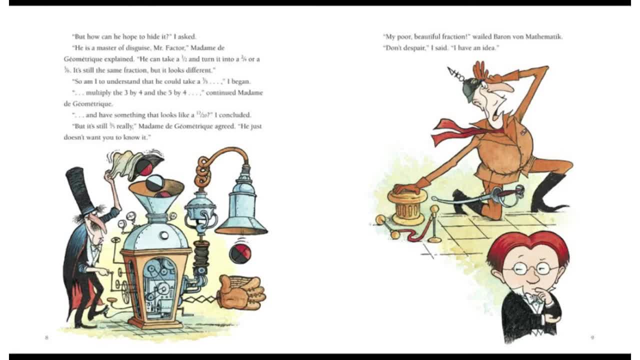 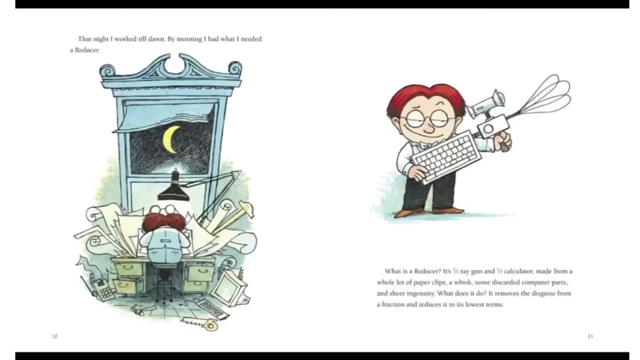 But it's still three-fifths really. Madame de Geometrique, agreed, He just doesn't want you to know it. My poor beautiful fraction wailed. Baron von Mathematik, Don't despair. I said I have an idea. 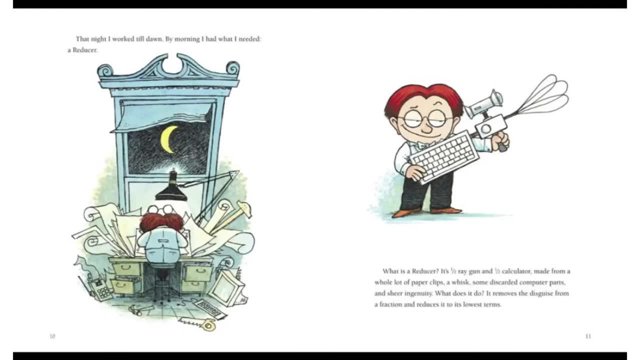 That night I worked till dawn. By morning I had what I needed: a reducer. What is a reducer? It's half ray gun and half calculator made from a whole lot of paper clips, a whisk, some discarded computer parts and sheer ingenuity. 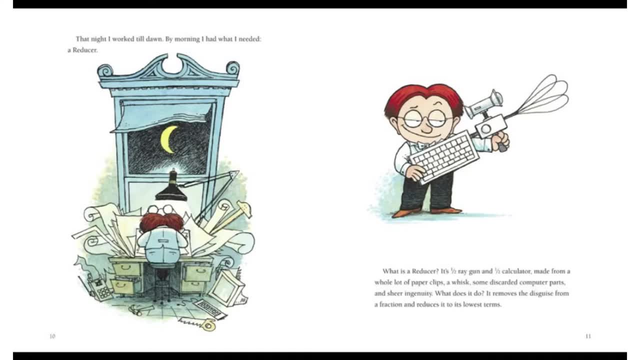 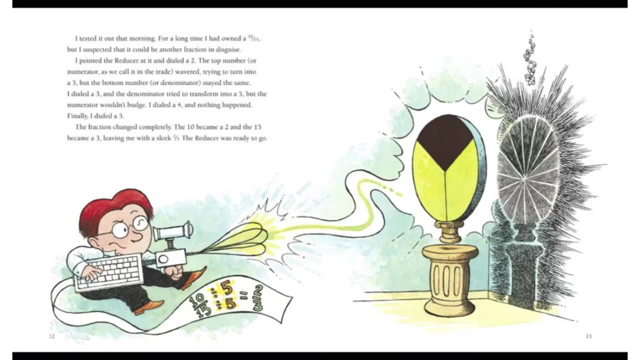 What does it do? It removes the disguise from a fraction and reduces it to its lowest terms. I tested it out that morning. For a long time I had owned a ten over fifteen, but I suspected that it could be another fraction in disguise. 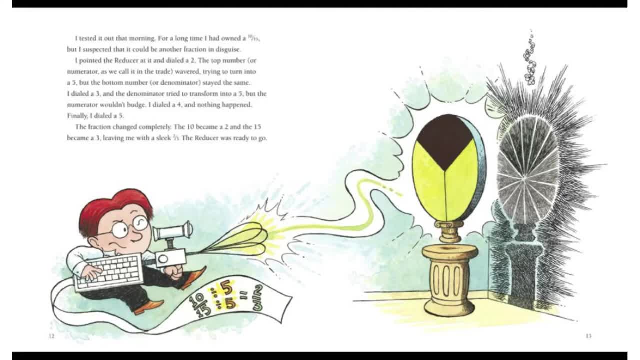 I pointed the reducer at it and dialed it in. It dialed a two, The top number wavered, trying to turn into a five, But the bottom number stayed the same. I dialed a three and the denominator turned to transform into a five, but the numerator 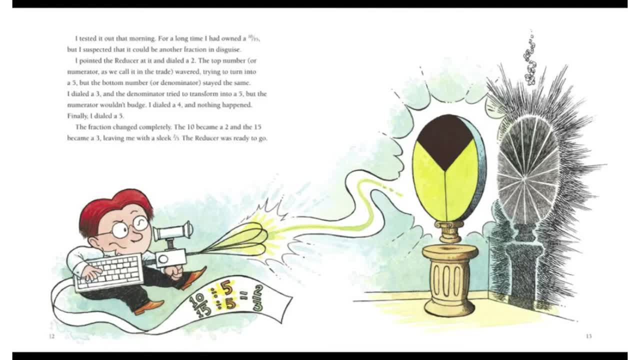 wouldn't budge. I dialed a four and nothing happened. Finally, I dialed a five. The fraction changed completely: The ten became a two and the fifteen became a three, leaving me with a sleek two-thirds words. The reducer was ready to go. 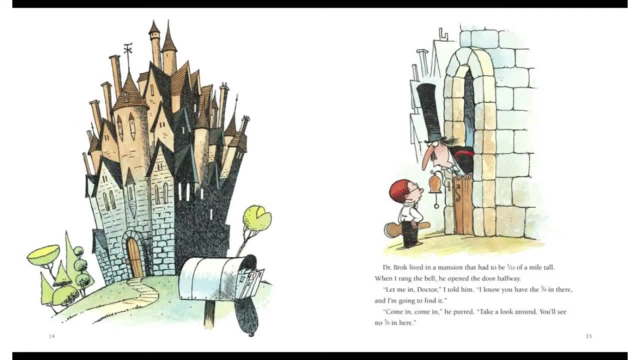 Doctor Brock lived in a mansion that had to be one tenth of a mile tall. When I rang the bell he opened the door half way. Let me in, Doctor. I told him. I know you have the Five Nights in there and I'm going to. 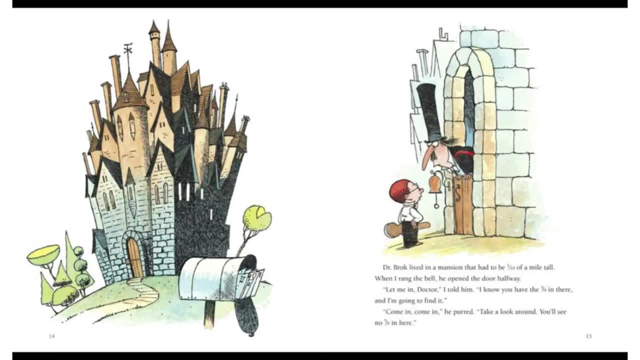 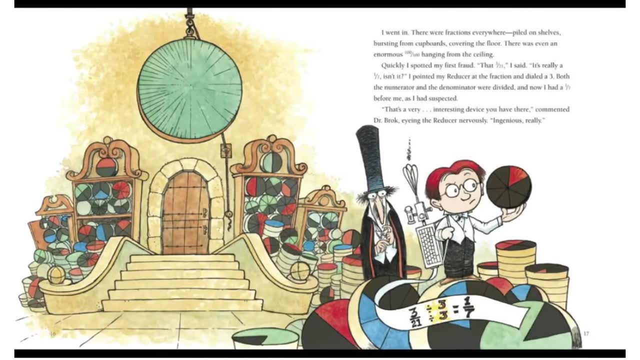 find it. Come in, come in, he purred. Take a look around, You'll see no. Five Nights in here. I went in. There were fractions everywhere piled on shelves, bursting from cupboards covering the floor. There was even an enormous one hundred one hundredths hanging from the 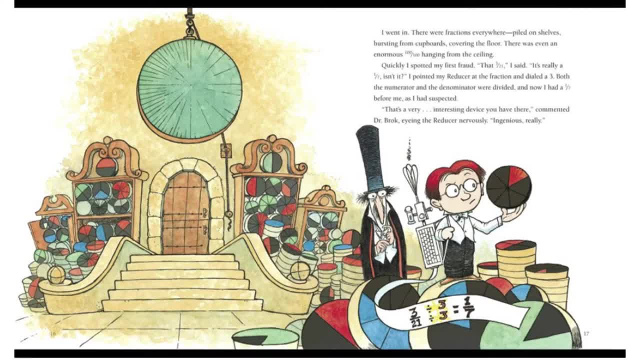 ceiling. Quickly I spotted my first fraud: That three over twenty-one. I said It's really one over seven, isn't it? I pointed my reducer at the fraction and dialed a three. Both the numerator and the denominator were divided and now I had a one-seventh. 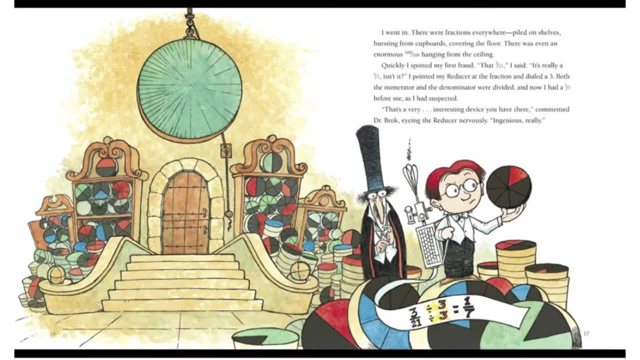 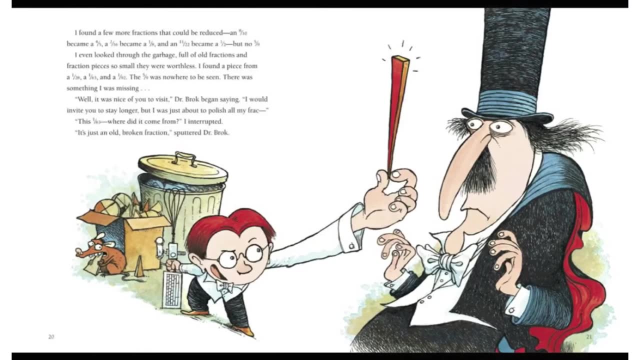 That's a very interesting device you have there, commented Doctor Brock, eyeing the reducer- nervously. Ingenious, really. I found a few more fractions that could be reduced: An eighteen over ten became a fourth over five, A twelve over sixteen became a one-eighth, and an eleven over twenty-two became 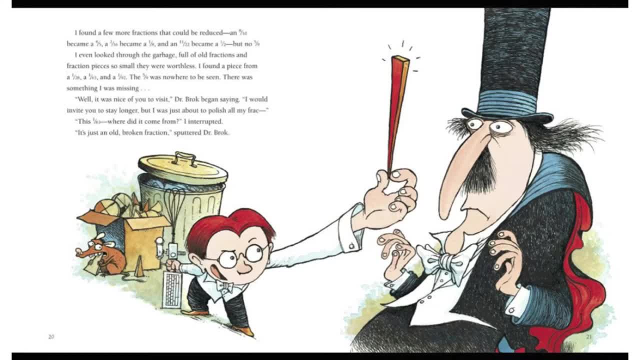 a half, But no Five Nights. I even looked through the garbage full of old fractions and fraction pieces, so small they were worthless. I found a piece from a one over twenty-eight, a one over sixty-three and a one over ninety-two. The Five Nights was nowhere to be seen There. 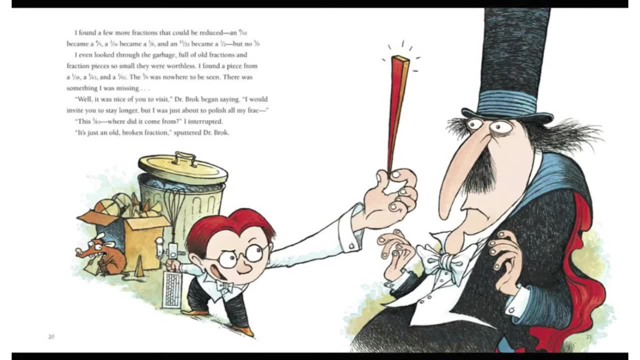 was something I was missing. Well, it was nice of you to visit. Doctor Brock began saying I would invite you to stay longer, but I was just about to polish all my frack. This one over sixty-three. where did it come from? I interrupted. 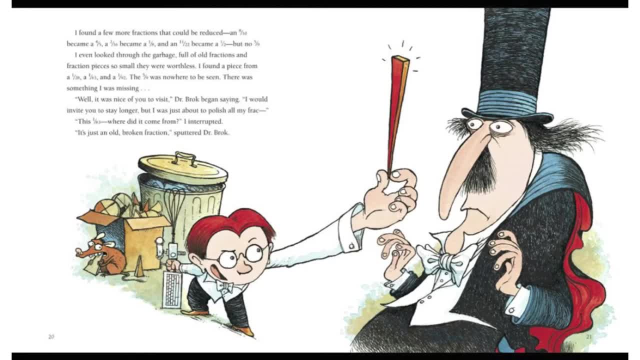 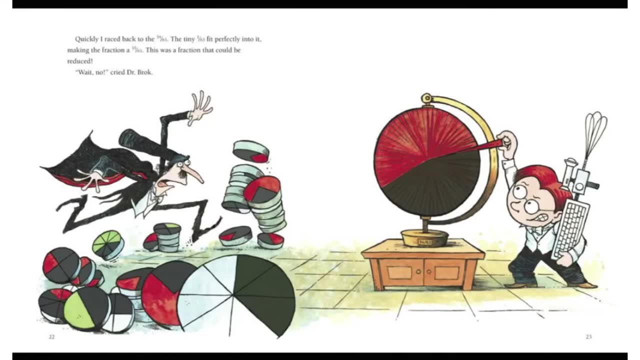 It's just an old b-b-broken fraction. sputtered Doctor Brock. Quickly I raced back to the thirty-four over sixty-three. The tiny one over sixty-three fit perfectly into it, making the fraction a thirty-five over sixty-three. This was a 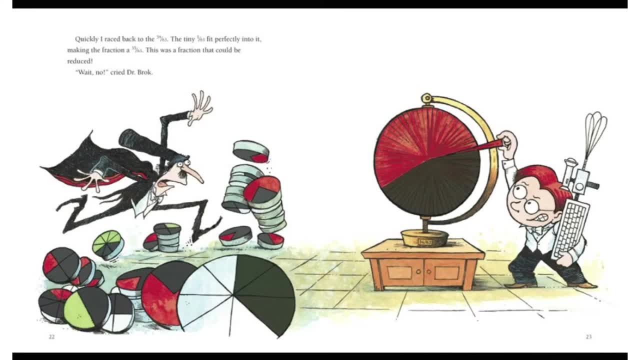 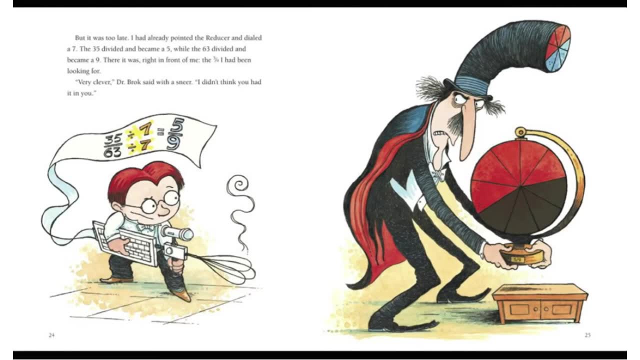 fraction that could be reduced. Wait no, cried Doctor Brock, But it was too late. I had already pointed the reducer and dialled the seven. The thirty-five divided and became a five, while the sixty-three divided and became a nine. There it was right. 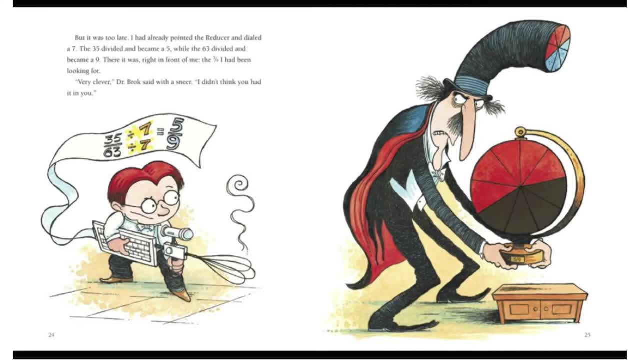 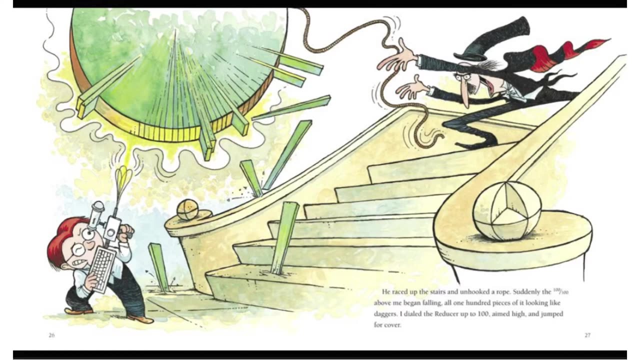 in front of me the Five Nights I had been looking for. Very clever Doctor Brock said with a sneer: I didn't think you had it in you. He raced up the stairs and unhooked a rocking chair rope. Suddenly the 100 over 100 above me began falling- all 100 pieces of it, looking like. 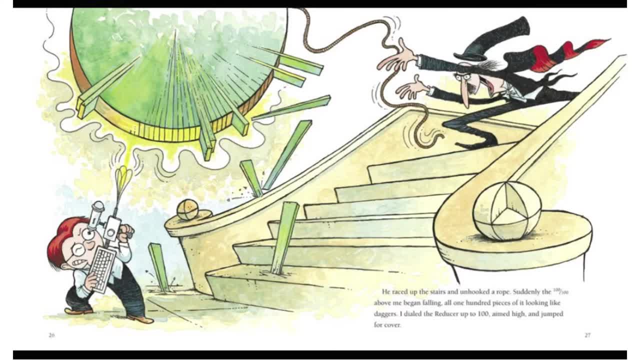 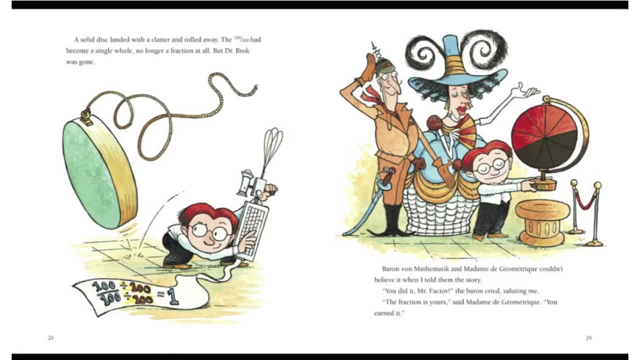 daggers. I dialed the reducer up to 100, aimed high and jumped for cover. A solid disc landed with a clatter and rolled away. The 100 over 100 had become a single hole, no longer a fraction at all. but Dr Brock was gone. 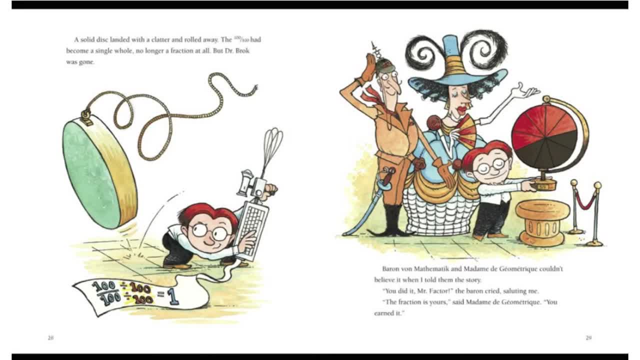 Hmm, Baron von Mathematik and Madame de Geometrique couldn't believe it when I told them the story. You did it, Mr Factor. the Baron cried, saluting me. The fraction is yours, said Madame de Geometrique. You earned it. I put it in the most prominent place on my top shelf. 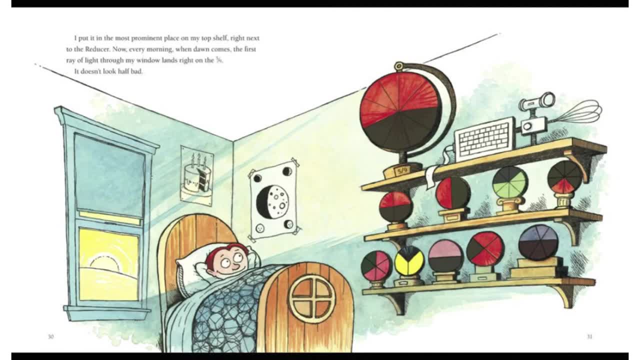 right next to the reducer. Now, every morning, when dawn comes, the first ray of light through my window lands right on top of it. I put it in the most prominent place on my top shelf. on the five nights It doesn't look half bad. 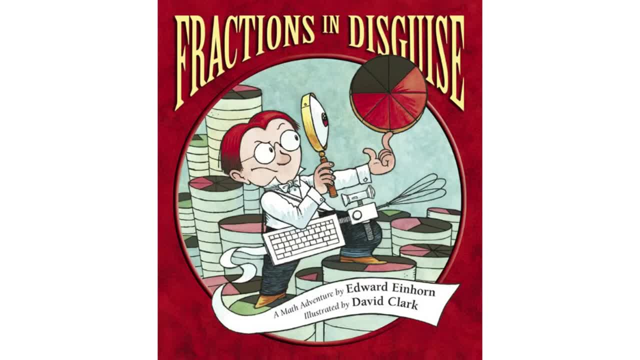 What did you think of this book? Fractions in Disguise? Let me know in the comments below and tune in next time.